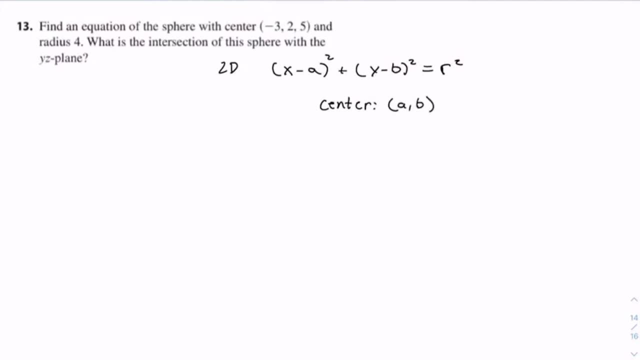 So, like most 2D formulas, we can build it off this in 3D. So, and we can just do that by adding one more component, say z minus c, squared Alright. so we have our point 3,, 2,, 5, which is our center point, and we can say a equals negative 3.. 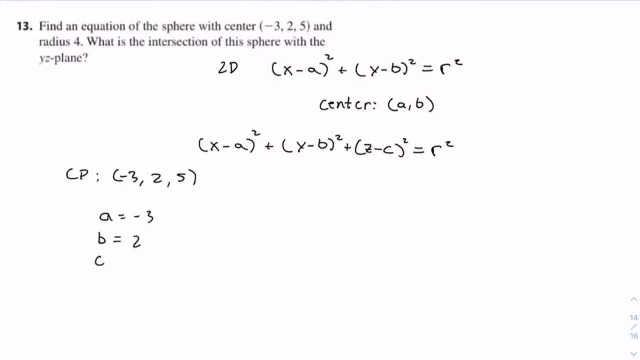 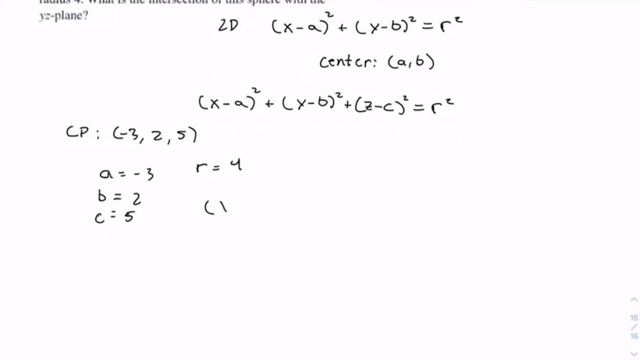 b equals 2,, c equals 5, and we have our radius r, which equals 4.. So we have x minus minus 3, which is plus 3, squared plus y minus 2, squared plus z minus 5 squared. 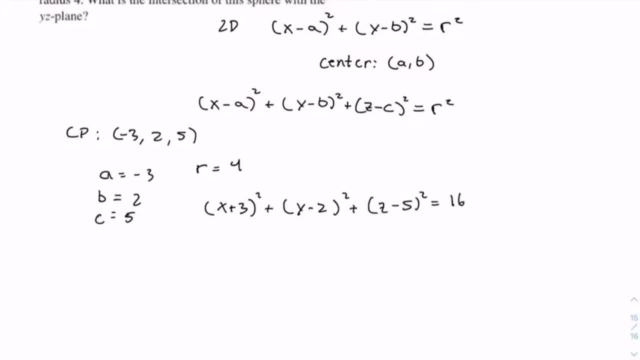 Equals 4 squared, which is 16.. So here's the equation of the sphere, with center negative 3,, 2, 5 and radius 4.. So now this is asking: what is the intersection of the sphere with the y z plane? 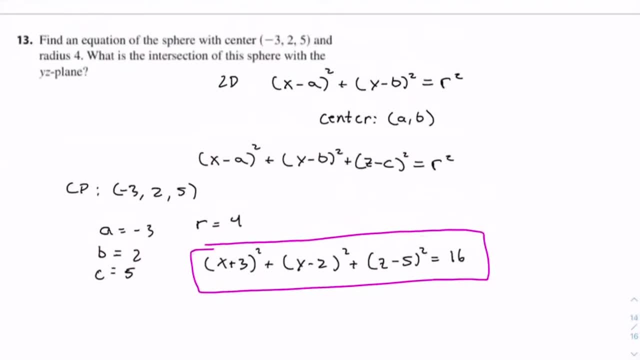 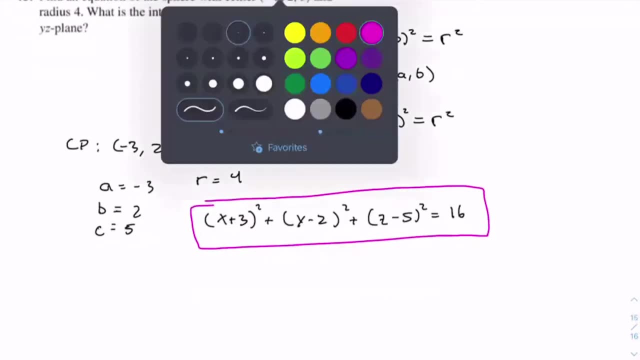 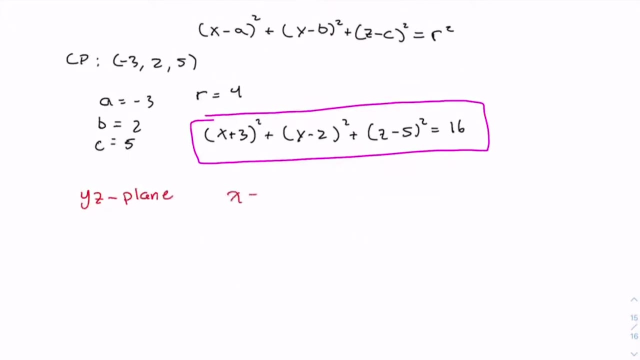 So there's a couple ways we can do this. We can draw it out and see what the sphere is. But we know that at the y z, We know that at the y z plane, we have the y z plane, x equals 0.. 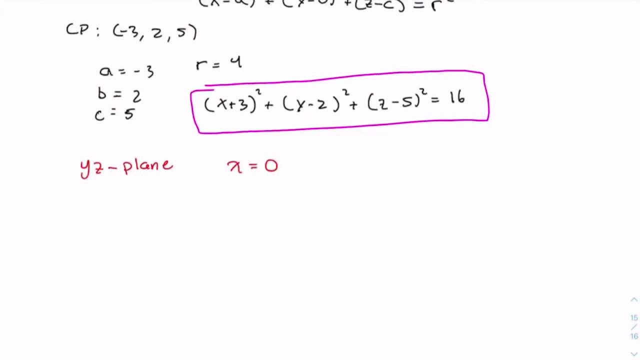 So if we just substitute x equals 0 to this equation, we have the intersection. So when x equals 0, we have 0 plus 3 squared, plus y minus 2 squared, plus z minus 5 squared, Equals 16.. 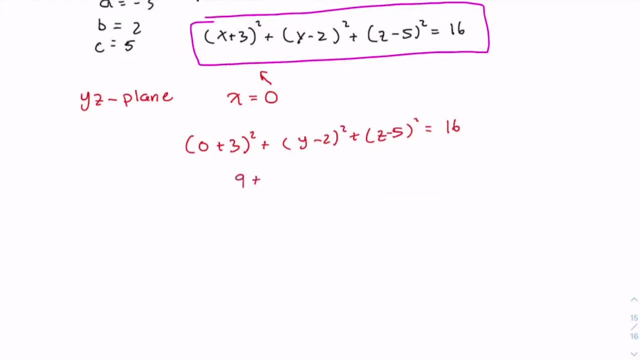 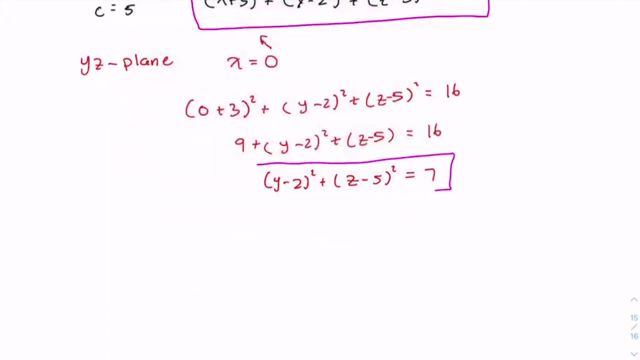 This is 9, plus all this stuff. So subtract 9 from both sides and we have y minus 2 squared plus z minus 5 squared equals 7.. So this is the intersection on the y- z plane. 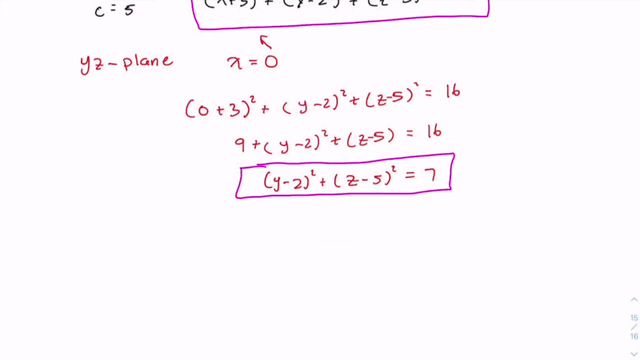 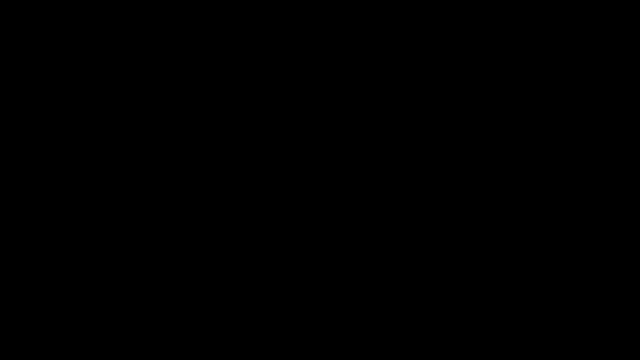 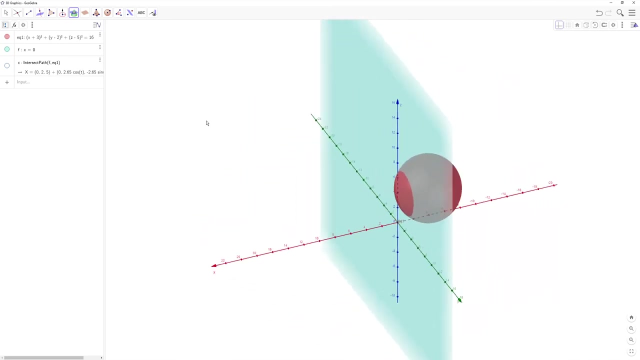 And to check this out on a graph, so we can visually see this, we can use a 3D graphing application And here we have our sphere graphed And we have our x, my bad, y, z plane.